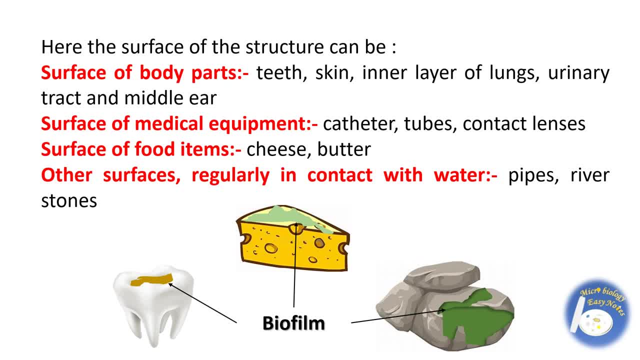 of body parts like teeth, skin, inner layer of lungs, urinary tract and middle layer. It can be surface of medical equipment like catheter, tubes, contact lenses. It can be surface of food items like cheese and butter- Other surfaces which are regularly in contact. 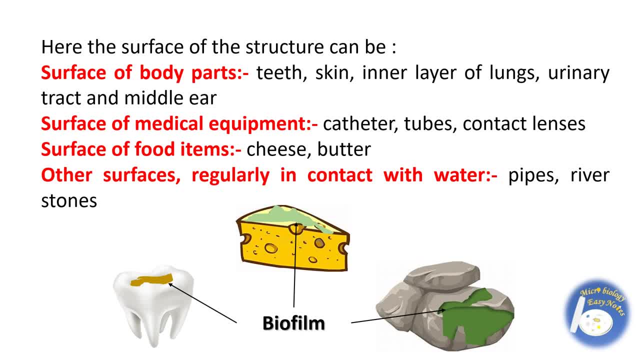 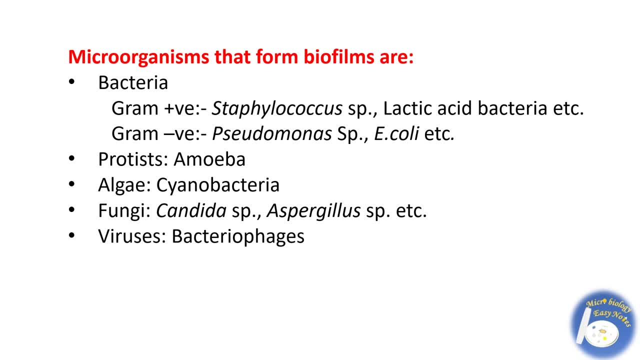 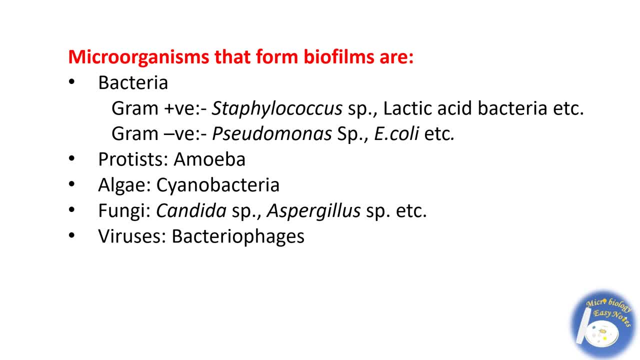 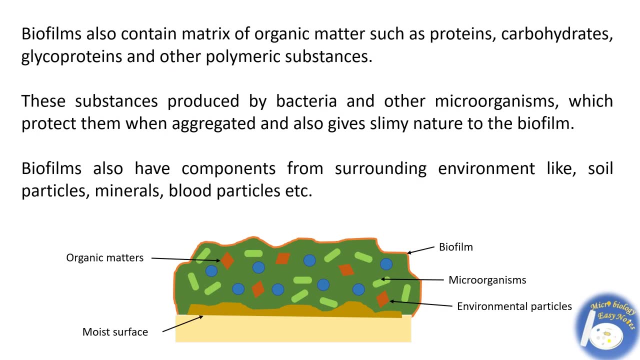 and Ecoli form biofilms. Protists like amoeba, algae like cyanobacteria, fungi such as Candida species and Aspergillus species. virus like bacteriophages also form biofilms. Biofilms also contain matrix of organic matters, such as proteins, carbohydrates, glycoproteins. 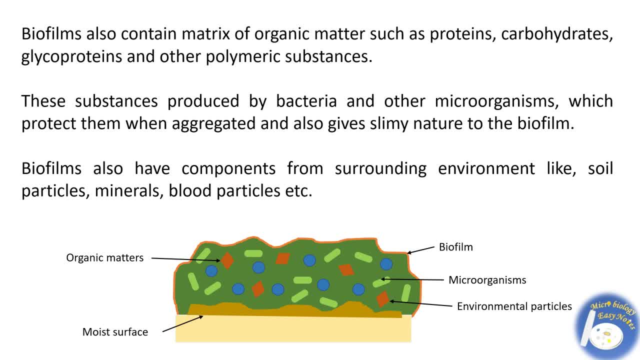 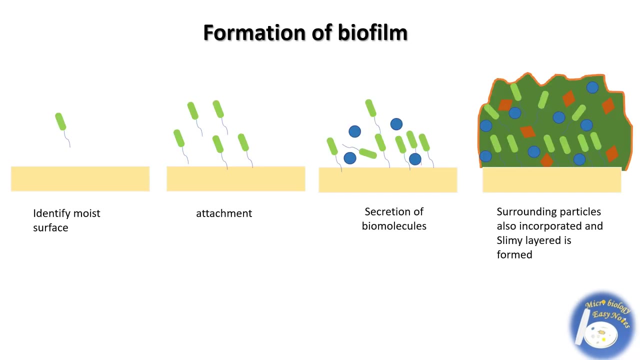 and other polymeric substances. These substances produced by bacteria and other microorganisms which protect them when aggregated and also gives slimy nature to the biofilm. Biofilms also have components from surrounding environment, like soil particles, minerals and blood particles, etc. Formation of Biofilm. 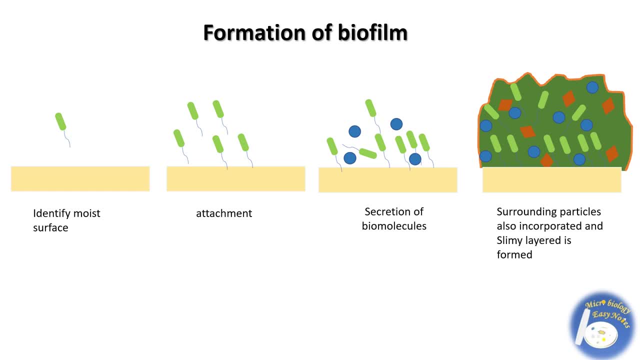 First, free-floating microorganisms attach to the surface. Using pilae, cells anchor themselves and adhere to the surface permanently. Cells secrete various biomolecules and create slimy structure around them for protection. This slimy structure, together with microorganisms, called biofilm. Biofilm also contains material from surrounding environment, like minerals. 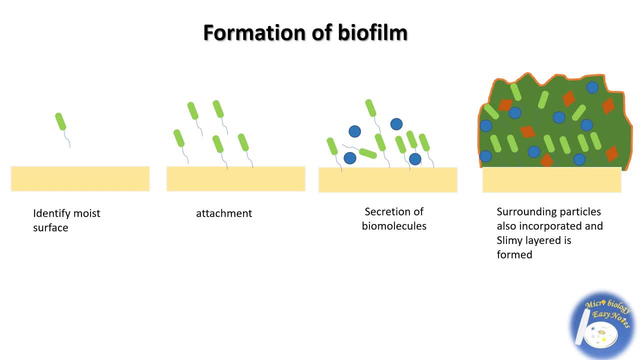 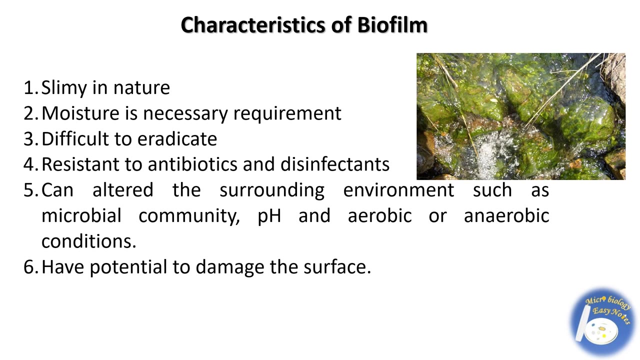 soil, particles and blood components, etc. It takes two days to form a biofilm And formation is not uniform. It may have various sizes and shapes. Characteristics of Biofilm: Biofilm is slimy in nature. Moisture is a necessary requirement to form a biofilm.